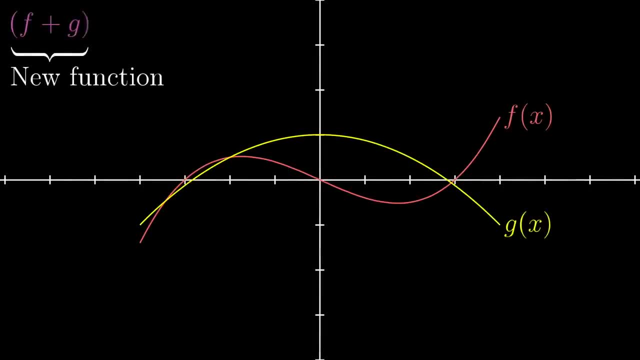 In the same way that you can add two vectors together, there's also a sensible notion for a new function, f and g, to get a new function, f plus g. It's one of those things where you kind of already know what it's going to be, but actually phrasing it is a mouthful. The output of this new function at any given input, like negative 4, is the sum of the outputs of f and g when you evaluate them each at that same input, negative 4. Or more generally, the value of the sum function at any given input x is the sum of the values f of x plus g of x. 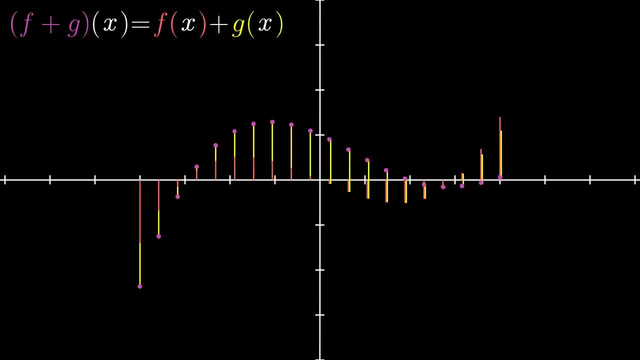 This is pretty similar to adding vectors coordinate by coordinate, it's just that there are, in a sense, infinitely many coordinates to deal with. 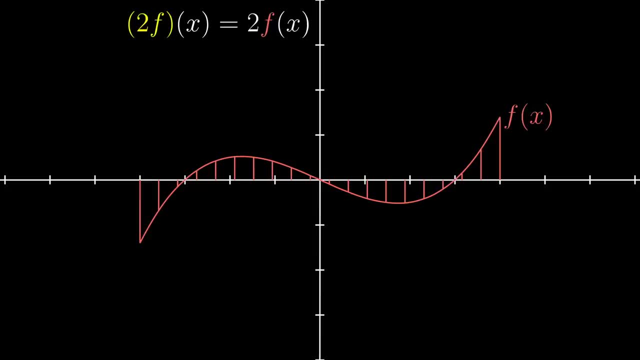 Similarly, there's a sensible notion for scaling a function by a real number. Just scale all of the outputs by that number. And again, this is analogous to scaling a vector, coordinate by coordinate. It just feels like there are infinitely many coordinates. 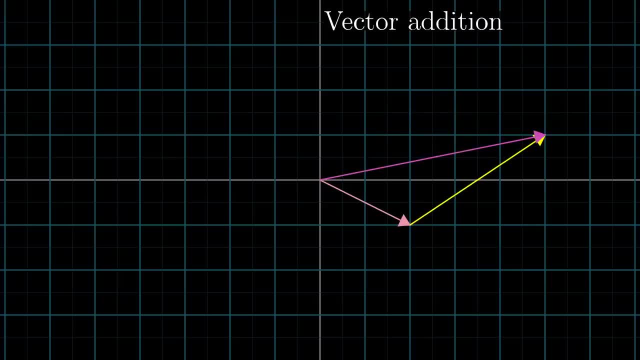 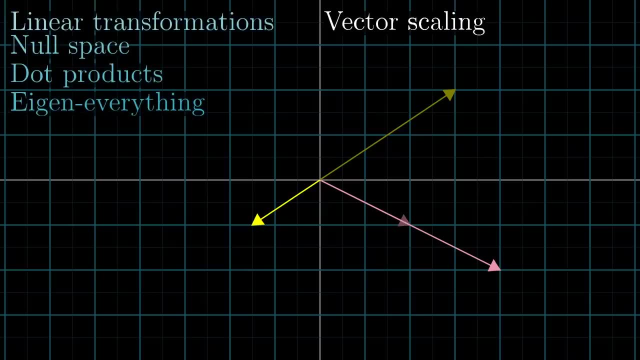 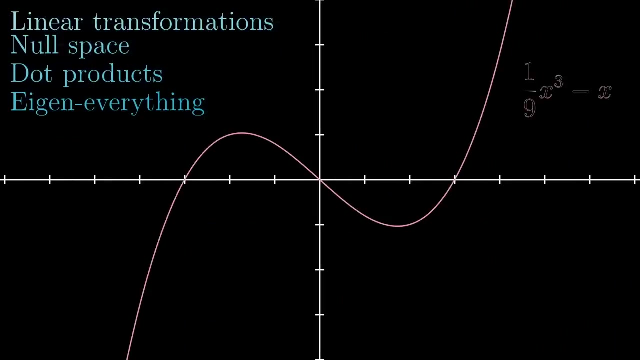 Now, given that the only thing vectors can really do is get added together or scaled, it feels like we should be able to take the same useful constructs and problem-solving techniques of linear algebra that were originally thought about in the context of arrows and space and apply them to functions as well. For example, there is a perfectly reasonable notion of a linear transformation for functions, something that takes in one function, and then has a function that takes in two functions. And then there's a perfectly reasonable notion of linear transformation for functions, something that takes in one function, and then has a function that takes in two functions. and turns it into another. 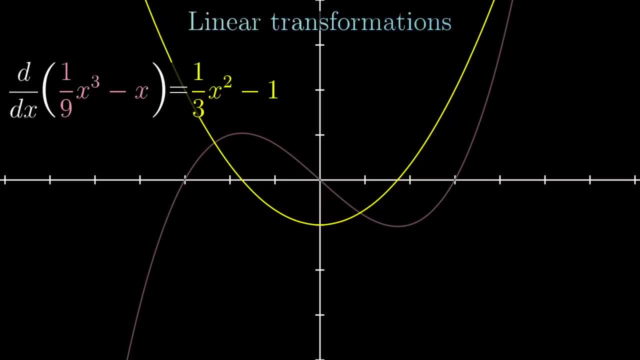 One familiar example comes from calculus, the derivative. 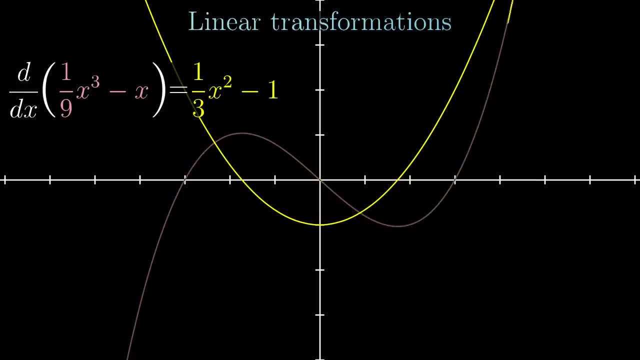 It's something which transforms one function into another function. 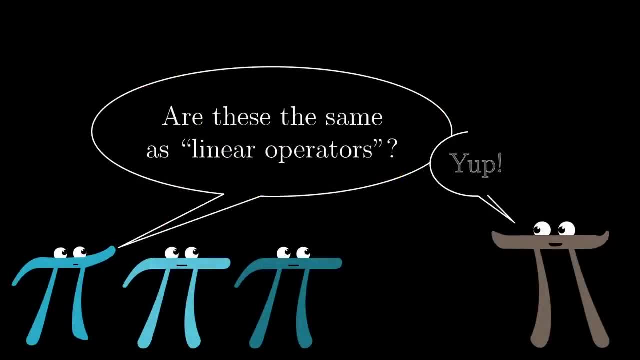 Sometimes in this context you'll hear these called operators instead of transformations, but the meaning is the same. 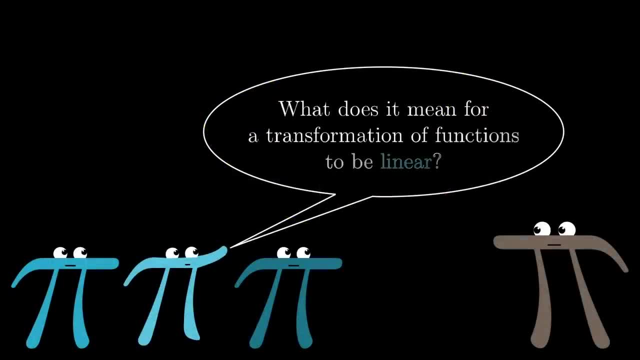 A natural question you might want to ask is what it means for a transformation of functions to be linear. 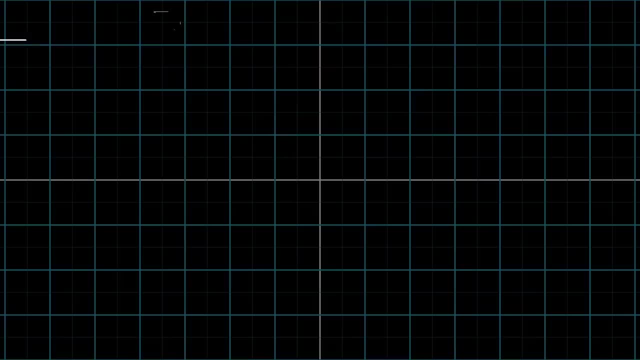 The formal definition of linearity is relatively abstract and symbolically driven compared to the way that I first talked about it in chapter three of this series. But the reward of abstractness is that we'll get something general enough to apply to functions as well as arrows. 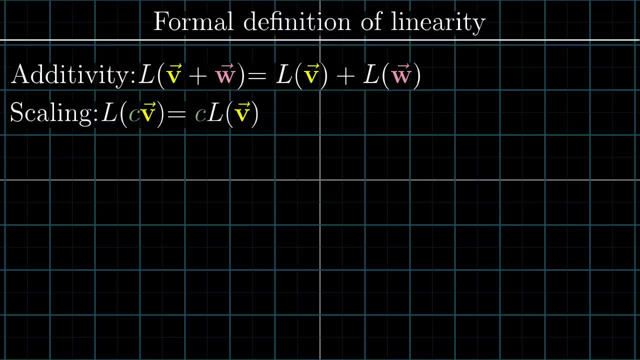 A transformation is linear if it satisfies two properties, commonly called additivity and scaling. 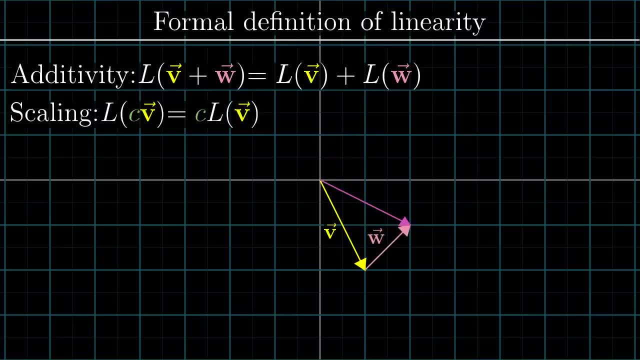 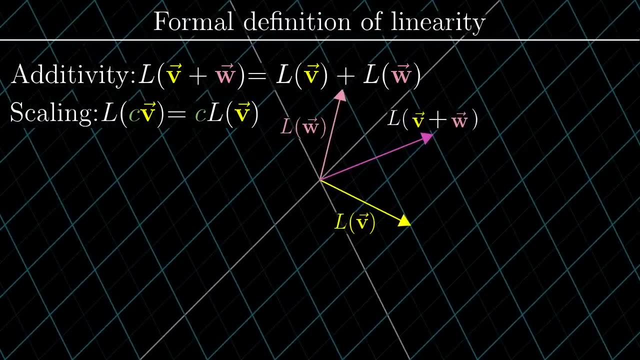 Additivity means that if you add two vectors, v and w, then apply a transformation to their sum, you get the same result as if you added the transformed versions of v and w. 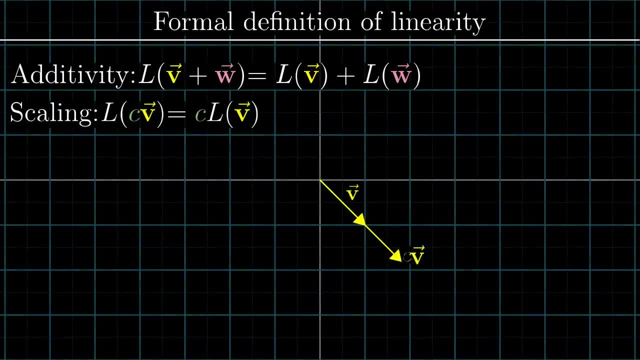 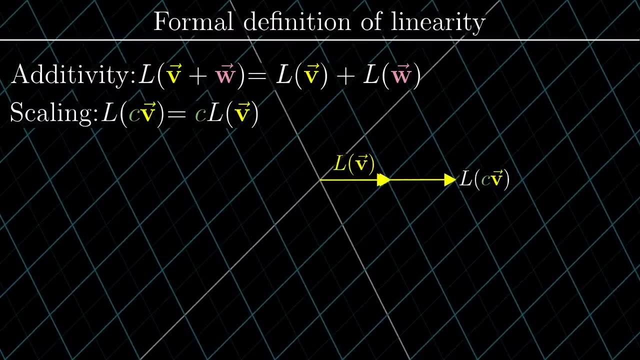 The scaling property is that when you scale a vector v by some number, then apply the transformation, you get the same ultimate vector as if you scaled the transformed version of v by that same amount. 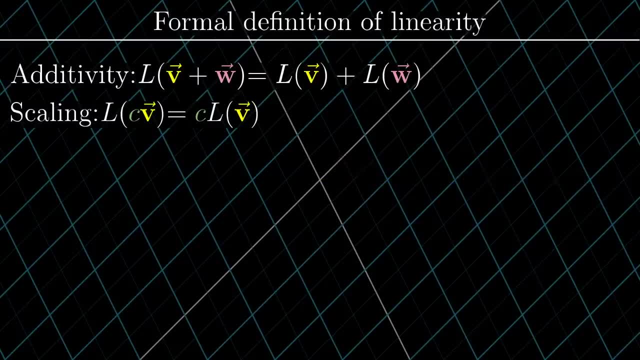 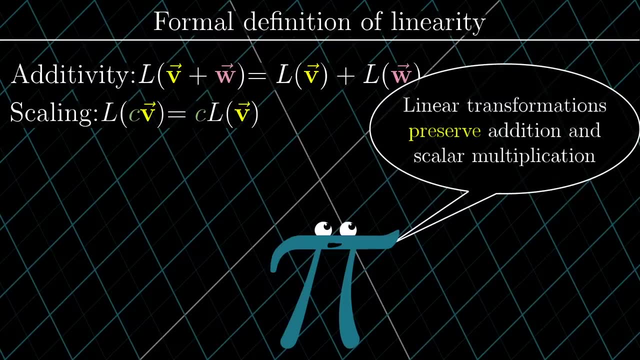 The way you'll often hear this described is that linear transformations preserve the operations of vector addition and scalar multiplication. 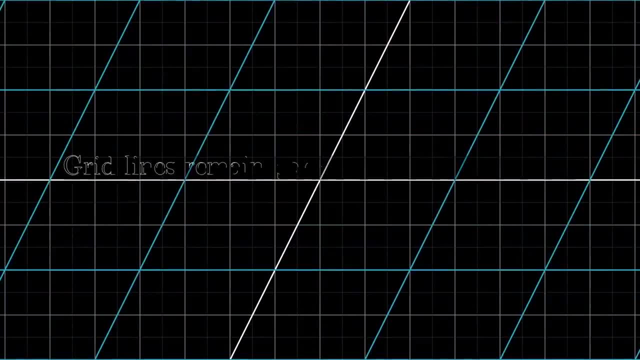 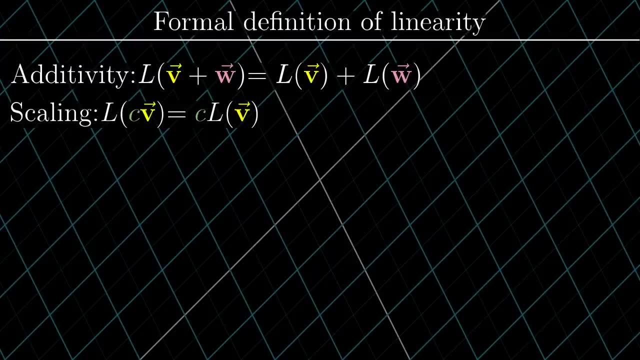 The idea of grid lines remaining parallel and evenly spaced that I've talked about in past videos is really just an illustration of what these two properties mean in the specific case of points in 2D space. 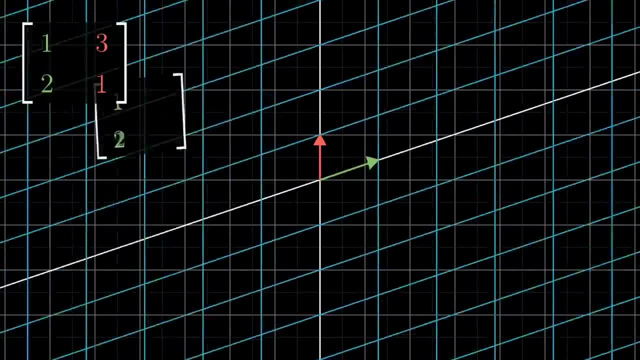 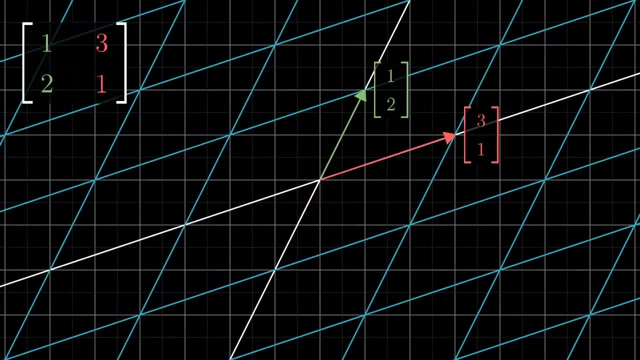 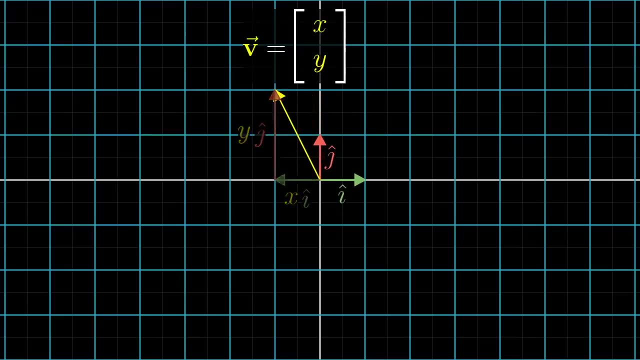 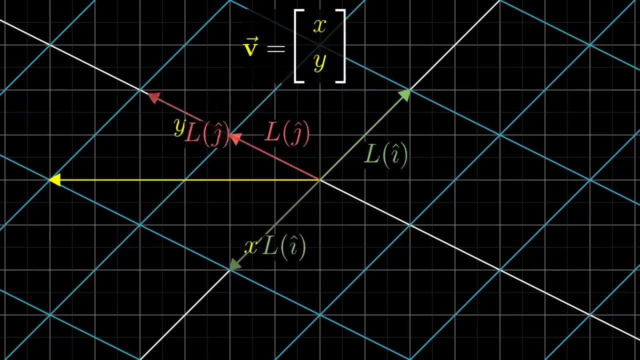 One of the most important consequences of these properties, which makes matrix vector multiplication possible, is that a linear transformation is completely described by where it takes the basis vectors. Since any vector can be expressed by scaling and adding the basis vectors in some way, finding the transformed version of a vector comes down to scaling and adding the transformed versions of the basis vectors in that same way. 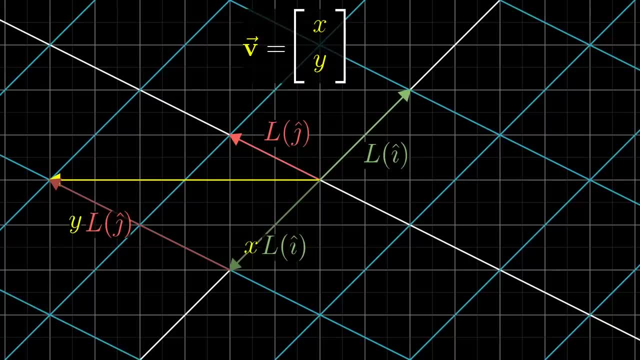 As you'll see in just a moment, this is as true for functions as it is for arrows. 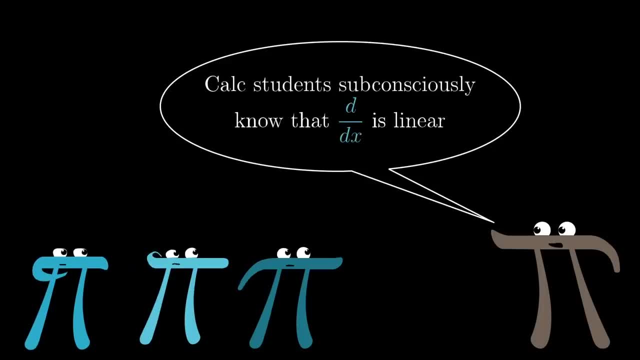 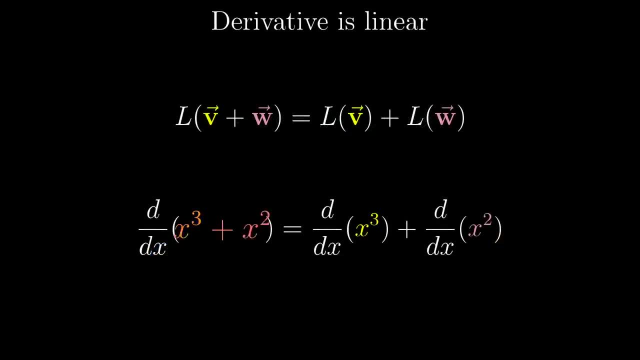 For example, calculus students, are always using the fact that the derivative is additive and has the scaling property, even if they haven't heard it phrased that way. If you add two functions, then take the derivative, it's the same as first taking the derivative of each one separately, then adding the result. 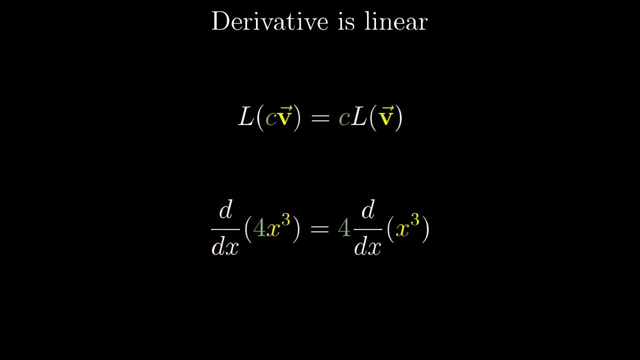 Similarly, if you scale a function, then take the derivative, it's the same as first taking the derivative, then scaling the result. 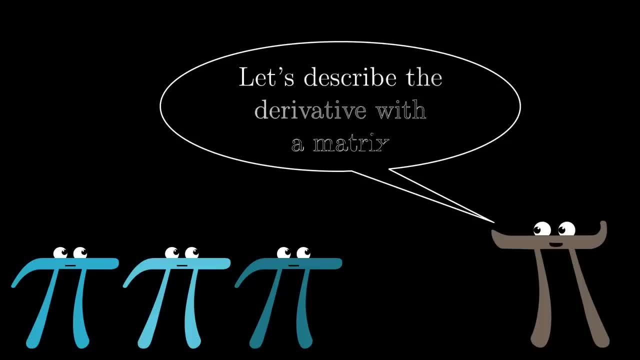 To really drill in the parallel, let's see what it might look like to describe the derivative with a matrix. This will be a little tricky, since function spaces have a tendency to be infinite dimensional, but I think this exercise is actually quite satisfying. 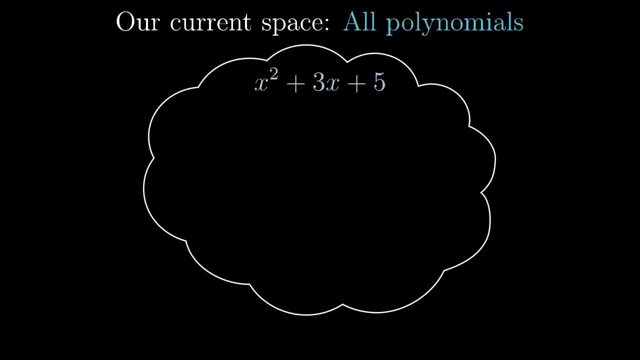 Let's limit ourself to polynomials, things like x squared plus three x plus five, or four x to the seventh minus five x squared. Each of the polynomials in our space will only have finitely many terms, but the full space is gonna include polynomials, 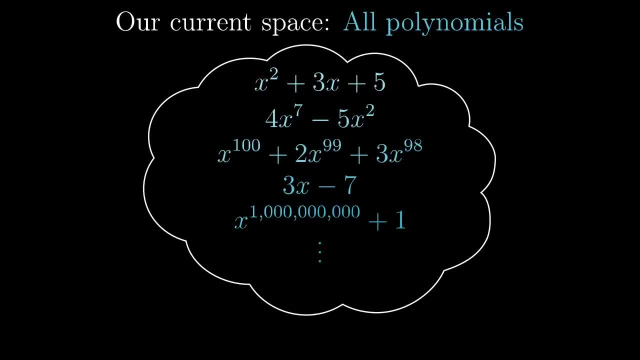 with arbitrarily large degree. The first thing we need to do is give coordinates to this space, which requires choosing a basis. 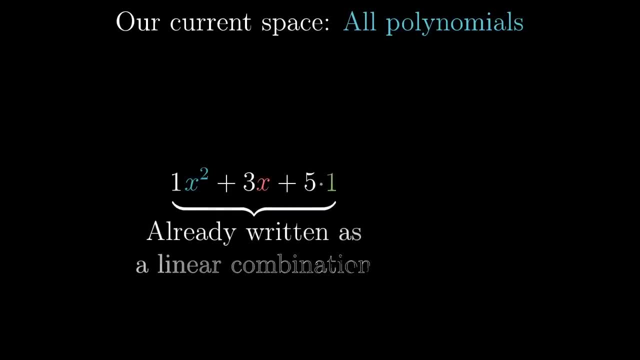 Since polynomials are already written down as the sum of scaled powers of the variable x, it's pretty natural to just choose pure powers of x as the basis function. In other words, our first basis function will be the constant function, b zero of x equals one. The second basis function will be b one of x equals x, then b two of x equals x squared, squared, then b3 of x equals x cubed, and so on. 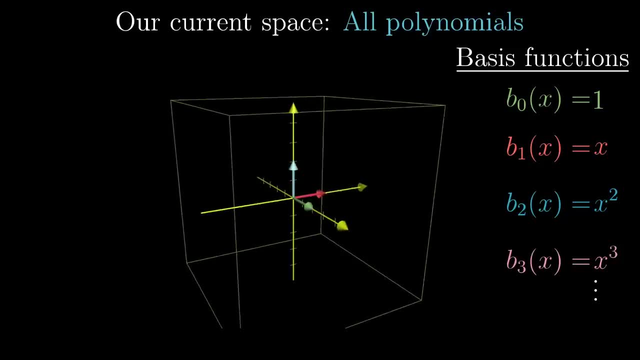 The role that these basis functions serve will be similar to the roles of i-hat, j-hat, and k-hat in the world of vectors as arrows. 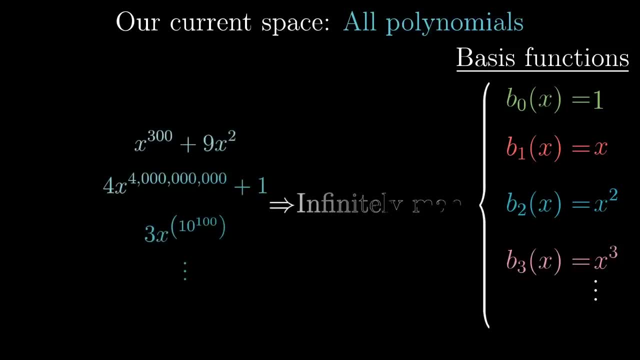 Since our polynomials can have arbitrarily large degree, this set of basis functions is infinite. 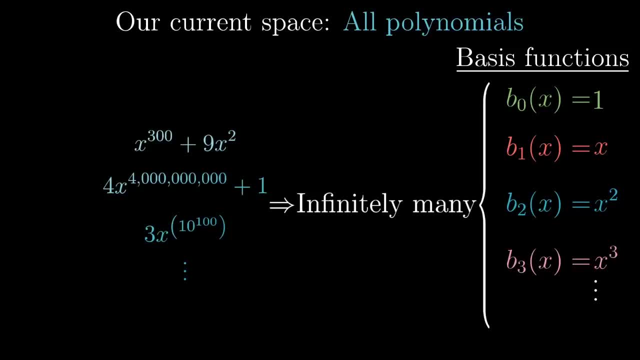 But that's okay, it just means that when we treat our polynomials as vectors, they're going to have infinitely many coordinates. A polynomial like x squared plus 3x plus 5, for example, would be described with the coordinates 5, 3, 1, then infinitely many zeros. You'd read this as saying that it's 5 times the first basis function, plus 3 times that second basis function, plus 1 times the third basis function, and then none of the other 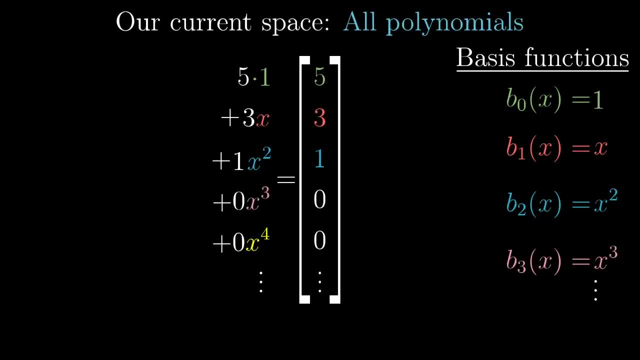 basis functions should be added from that point on. 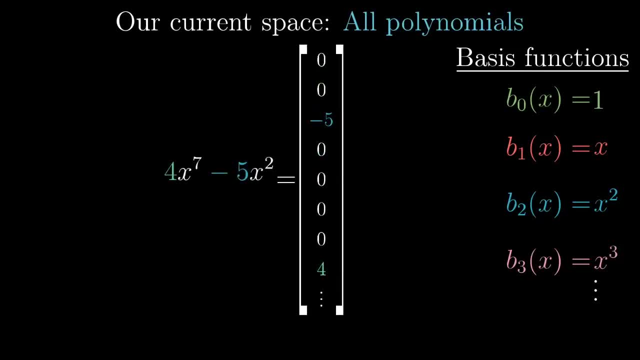 The polynomial 4x to the 7th minus 5x squared would have the coordinate 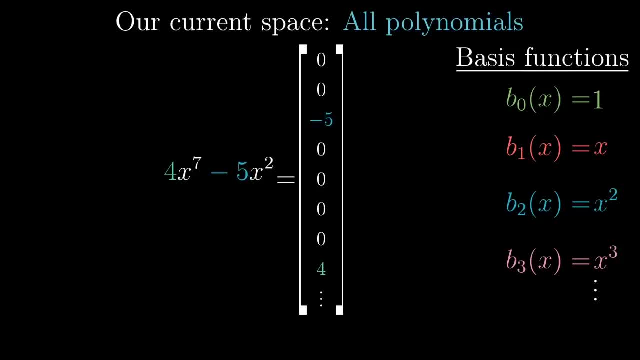 0, 0, negative 5, 0, 0, 0, 0, 4, then an infinite string of zeros. In general, since every individual polynomial has only finitely many terms, its coordinates will be some finite string of numbers with an infinite tail of zeros. 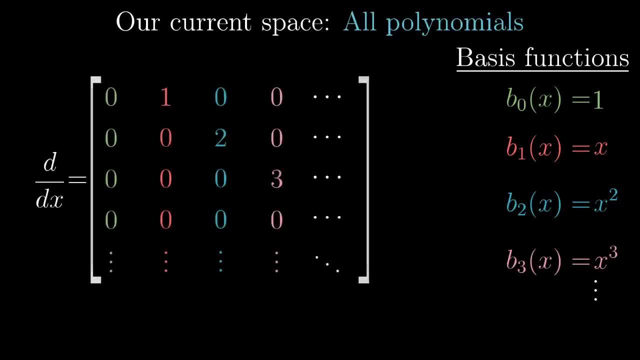 In this coordinate system, the derivative is described with an infinite matrix that's mostly full of zeros, but which has the positive integers counting down on this offset diagonal. I'll talk about how you could find this matrix in just a moment, but the best way to get a feel for it is to just watch it in action. 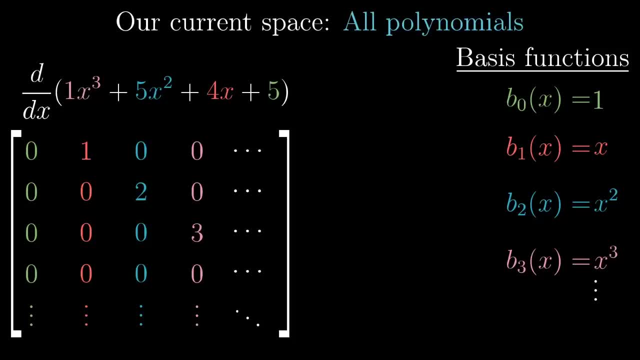 Take the coordinates representing the polynomial x cubed plus 5x squared plus 4x plus 5. Then put those coordinates on the right of the matrix. The only term that contributes to the first coordinate of the result is 1 times 4. Which means the constant term in the result will be 4. This corresponds to the fact that the derivative of 4x is the constant 4. The only term contributing to the second coordinate of the matrix vector product is 2 times 5. Which means the coefficient in front of x in the derivative is 10. That one corresponds to the derivative of 5x squared. Similarly, the third coordinate in the matrix vector product comes down to taking 3 times 1. 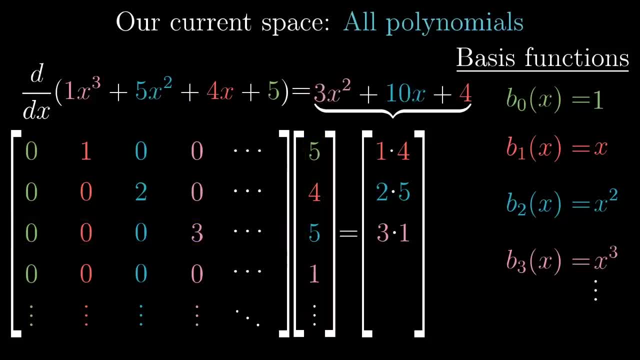 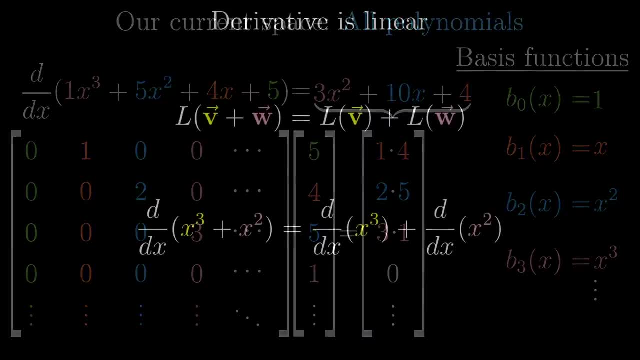 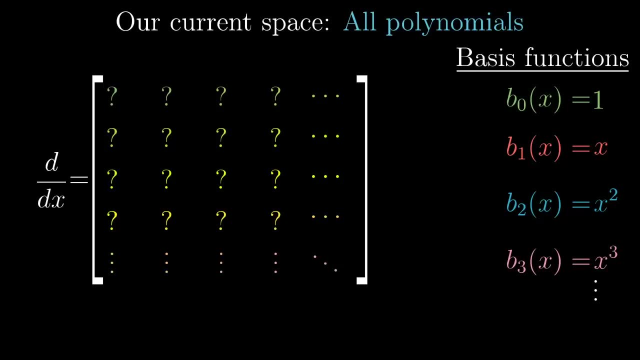 This one corresponds to the derivative of x cubed being 3x squared. And after that, it'll be nothing but zeros. What makes this possible is that the derivative is linear. And for those of you who like to pause and ponder, you could construct this matrix by taking the derivative of each basis function and putting the coordinates of the results in each column. 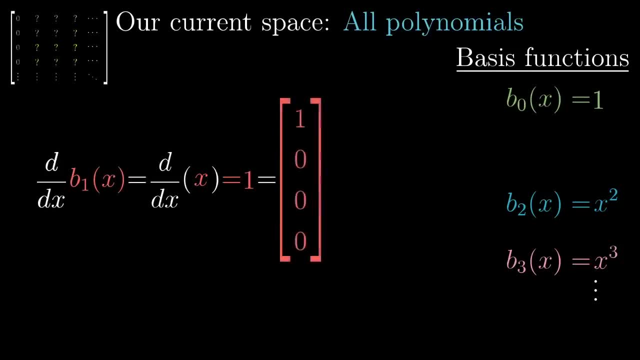 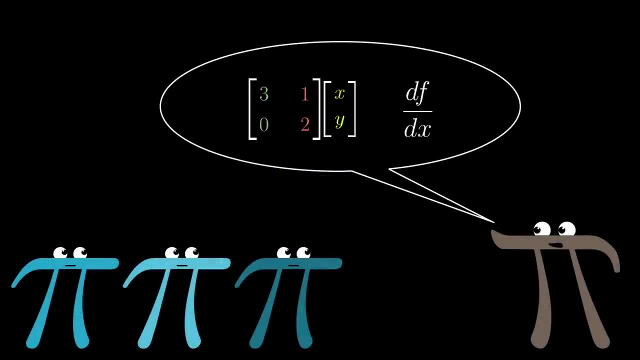 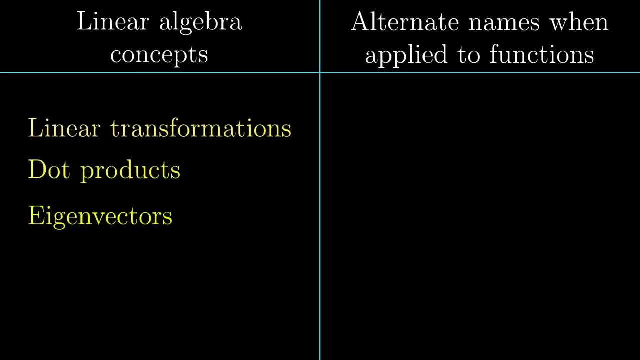 So, surprisingly, matrix-vector multiplication and taking a derivative, which at first seem like completely different animals, are both just really members of the same family. In fact, most of the concepts I've talked about in this series with respect to vectors as arrows in space, things like the dot product or eigenvectors, have direct analogs in the world of functions, though sometimes they go by different names, things like inner product or eigenfunction. 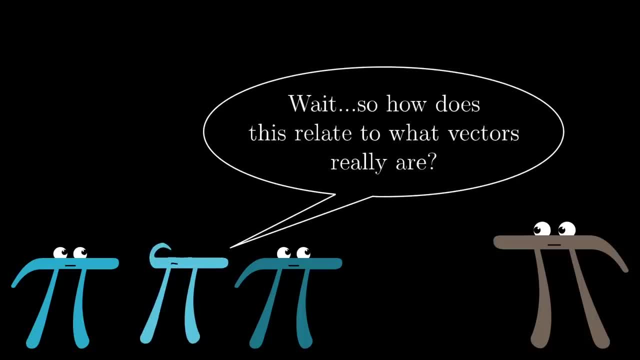 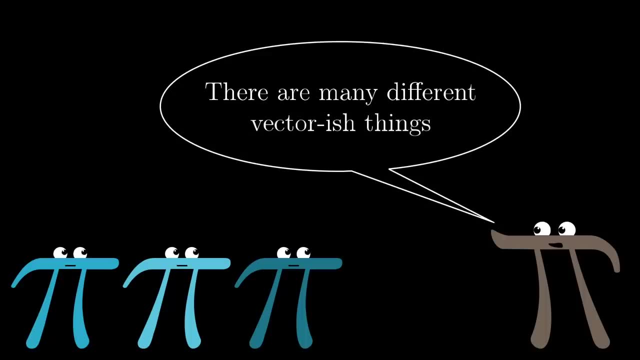 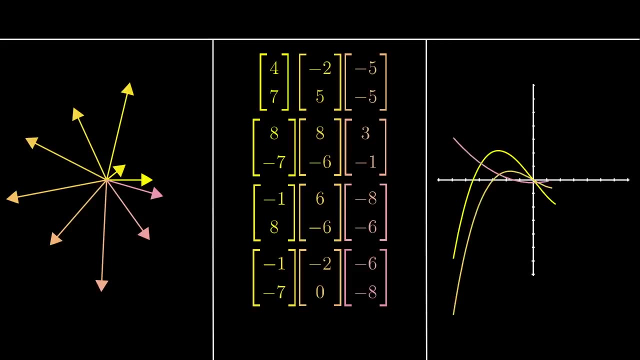 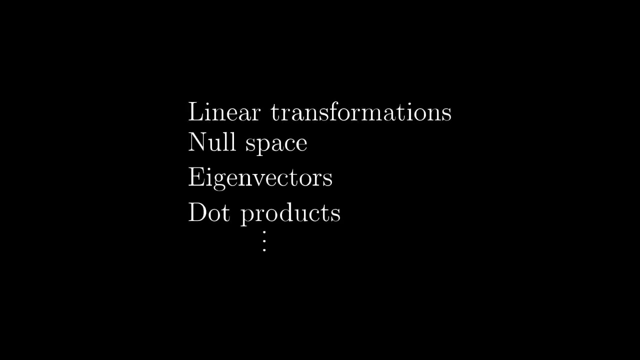 So back to the question of what is a vector. The point I want to make here is that there are lots of vector-ish things in math. As long as you're dealing with a set of objects where there's a reasonable notion of scaling and adding, whether that's a set of arrows in space, lists of numbers, functions, or whatever other crazy thing you choose to define, all of the tools developed in linear algebra regarding vectors, linear transformations and all that stuff, should be able to apply. Take a moment to imagine yourself right now as a mathematician developing the theory of linear algebra. 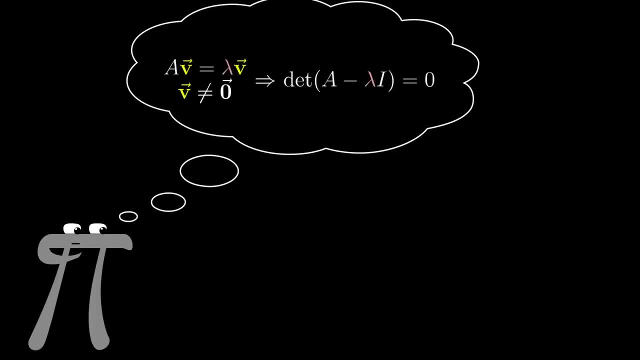 You want all of the definitions and discoveries of your work to apply to all of the vector-ish things in full generality, not just to one specific case. 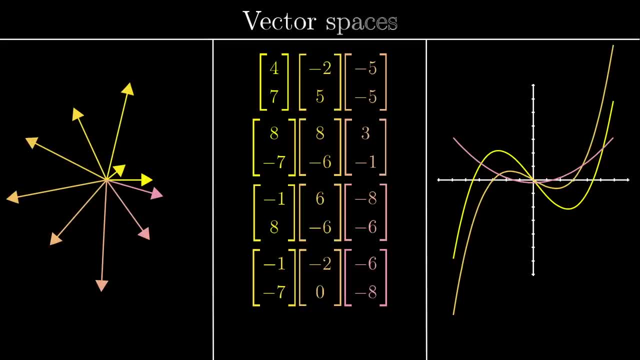 These sets of vector-ish things, like arrows or lists of numbers or functions, are called vector spaces. 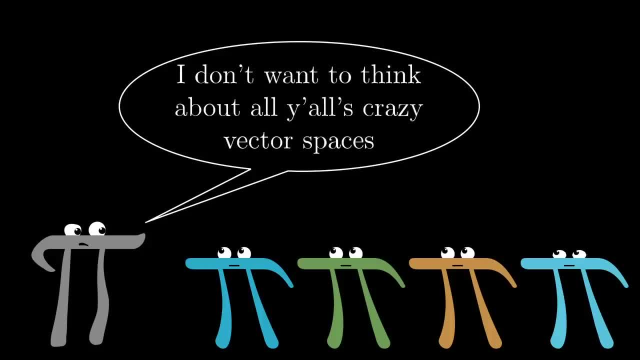 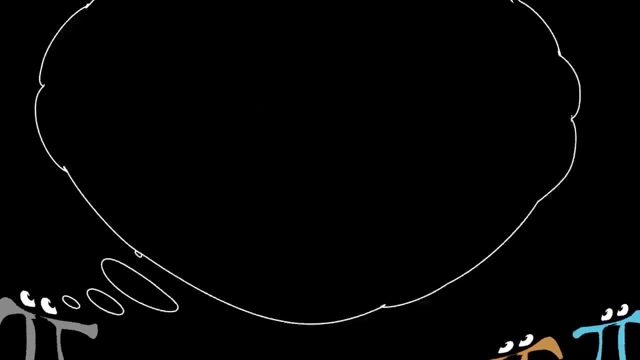 And what you as the mathematician might want to do is say, hey everyone, I don't want to have to think about all the different types of crazy vector spaces that y'all might come up with. So what you do is establish a list of rules that vector addition and scaling have to abide by. 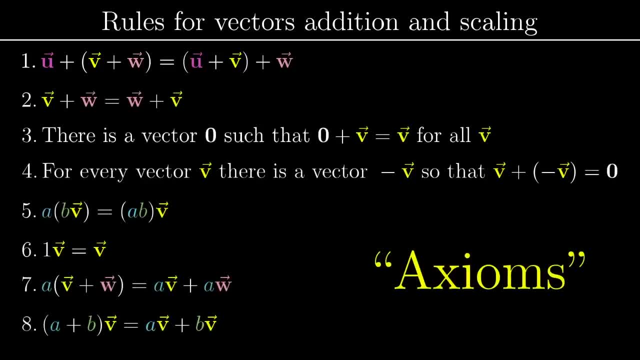 These rules are called axioms. And in the modern theory of linear algebra, there are eight axioms that any vector space must satisfy. 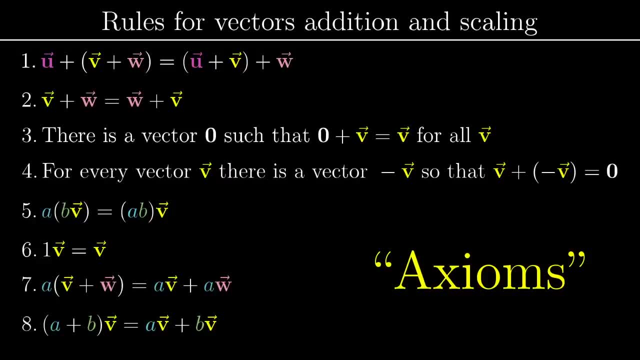 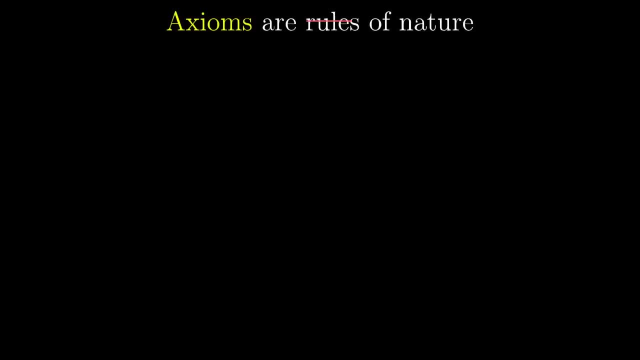 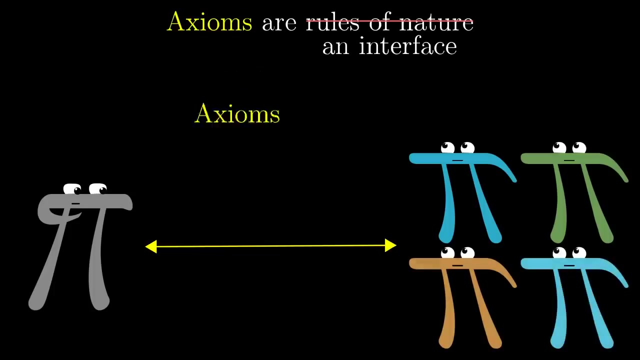 If all of the theory and constructs that we've discovered are going to apply. I'll leave them on the screen here for anyone who wants to pause and ponder, but basically it's just a checklist to make sure that the notions of vector addition and scalar multiplication do the things that you'd expect them to do. These axioms are not so much fundamental rules of nature as they are an interface between you, the mathematician discovering results, and other people who might want to apply those results to new sorts of vector spaces. 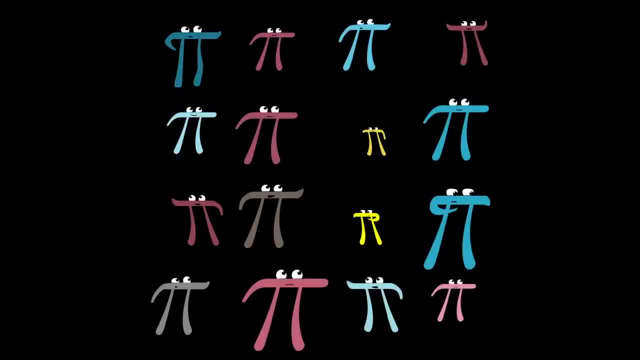 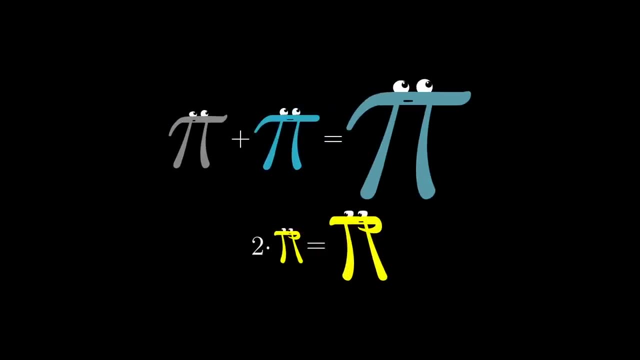 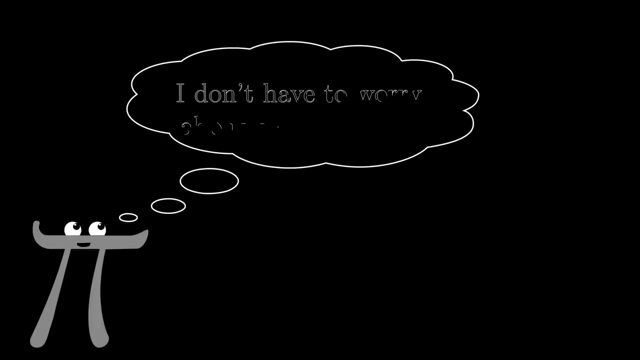 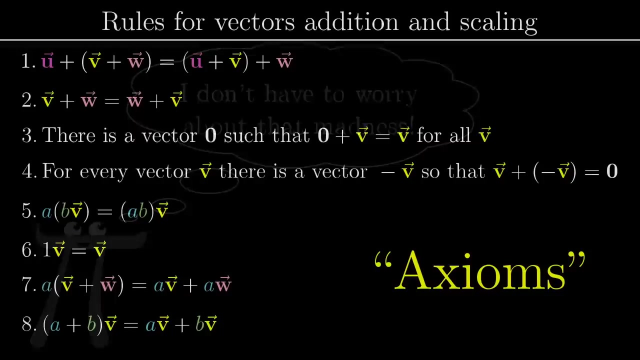 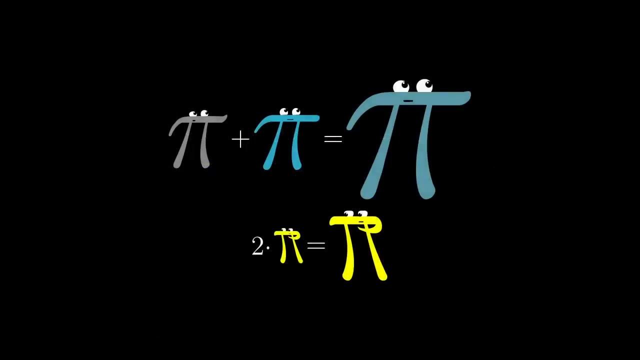 If, for example, someone defined some crazy type of vector space, like the set of all pi creatures with some definition of adding and scaling pi creatures, these axioms are like a checklist of things that they need to verify about their definitions before they can start applying the results of linear algebra. And you, as the mathematician, never have to think about all the possible crazy vector spaces people might define. You just have to prove your results in terms of these axioms, so anyone whose definitions satisfy those axioms can happily apply your results. Even if you don't have the knowledge to do that. 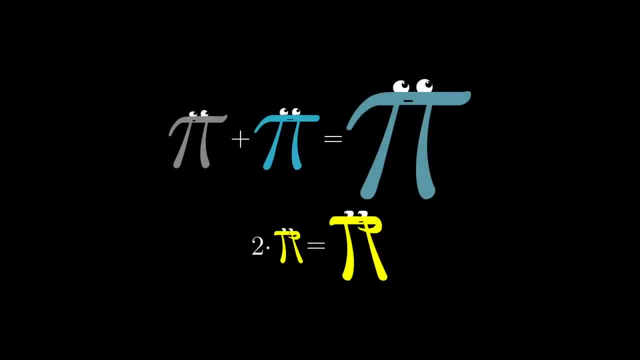 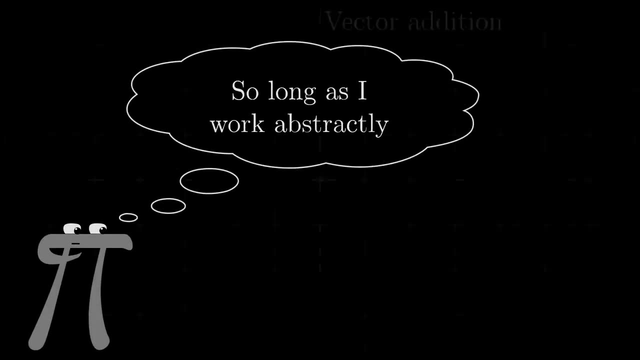 You never thought about their situation. As a consequence, you'd tend to phrase all of your results pretty abstractly, which is to say, only in terms of these axioms, rather than centering on a specific type of vector, 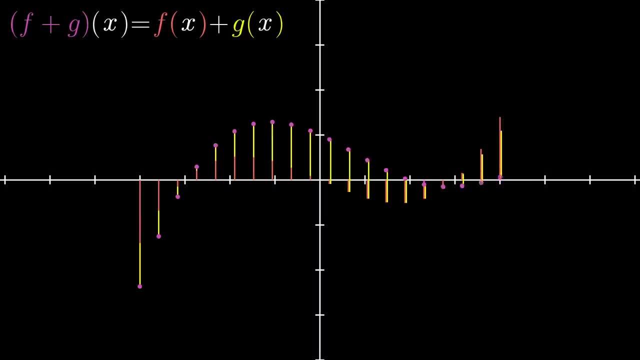 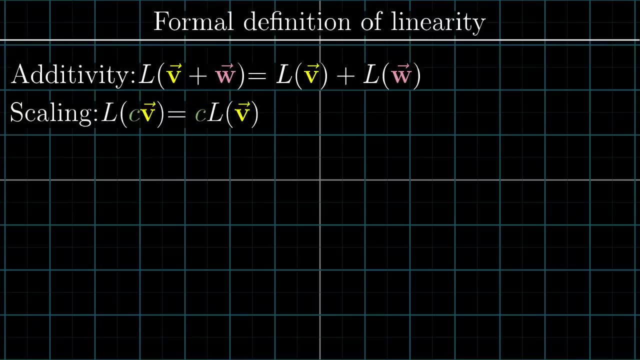 like arrows in space or functions. For example, this is why just about every textbook you'll find will define linear transformations in terms of additivity and scaling, rather than talking about gridlines remaining parallel and evenly spaced. 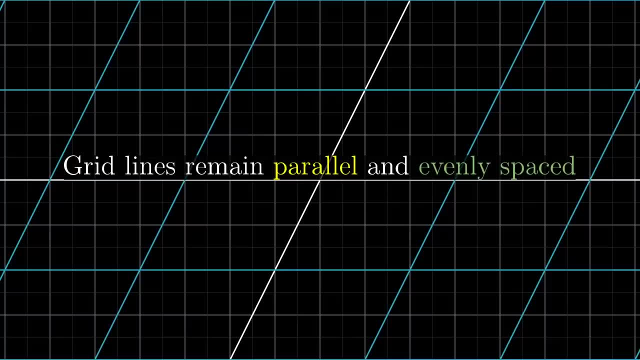 Even though the latter is more intuitive, and, at least in my view, more helpful for first-time learners, even if it is specific to one situation. 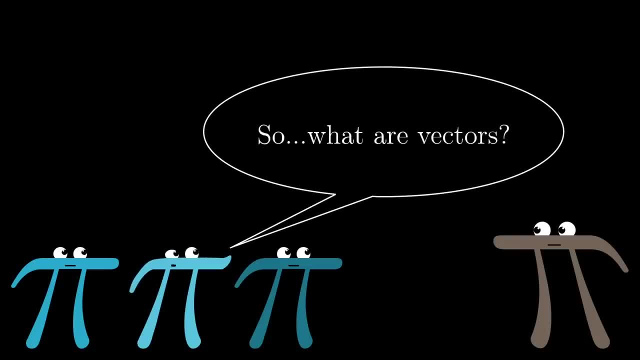 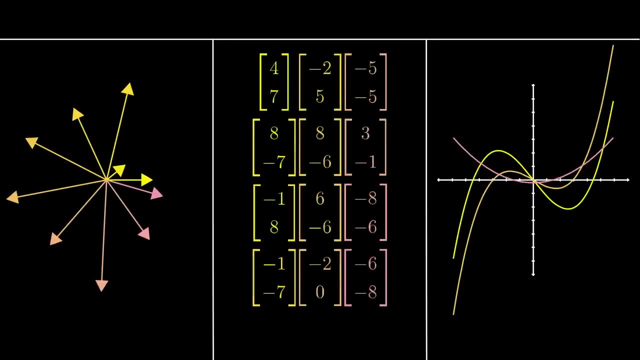 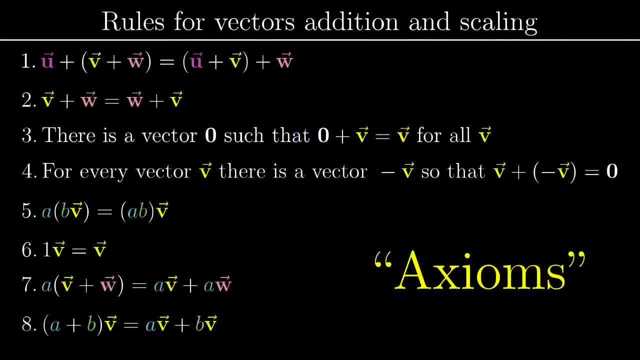 So the mathematician's answer to what are vectors is to just ignore the question. In the modern theory, the form that vectors take doesn't really matter. Arrows, lists of numbers, functions, pi creatures, really, it can be anything, so long as there is some notion of adding and scaling vectors that follows these rules. It's like asking what the number is. 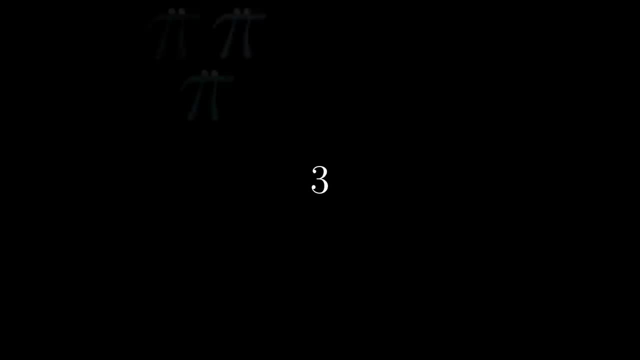 It's like asking what the number 3 really is. Whenever it comes up concretely, it's in the context of some triplet of things, but in math, it's treated as an abstraction for all possible triplets of things, and lets you reason about all possible triplets using a single idea. 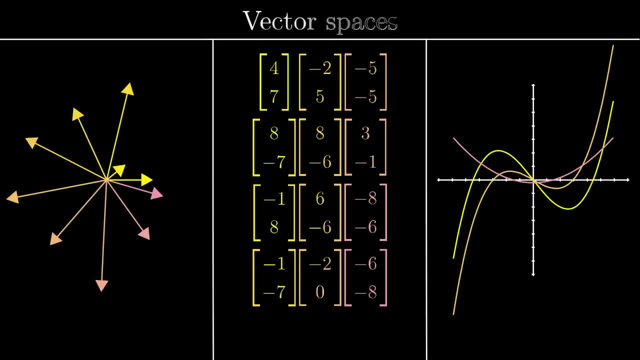 Same goes with vectors, which have many embodiments, but math abstracts them all into a single intangible notion of a vector space. 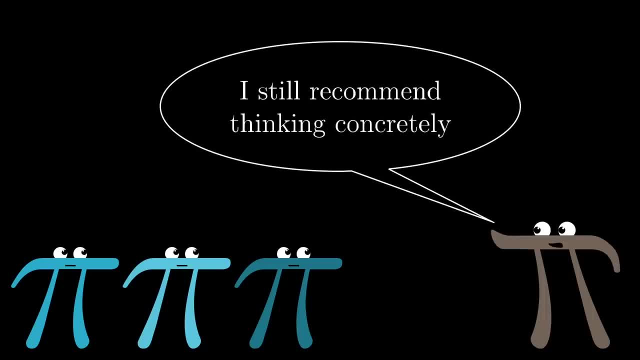 But as anyone watching this series knows, I think it's better to begin with the idea of a vector space in a concrete, visualizable setting, like 2D space, with arrows rooted at the origin.